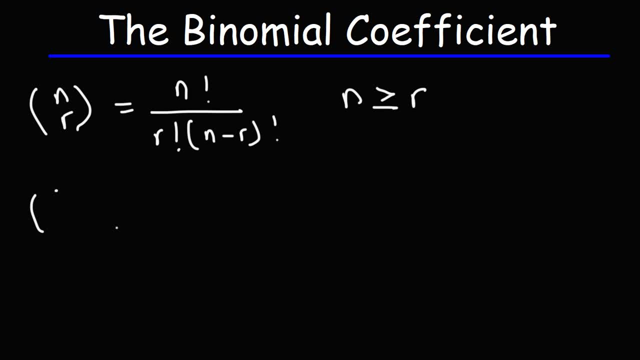 Let's say we have this expression: a 8 above 3.. Go ahead and evaluate that. So, using the formula, we can see that n is 8 and r is 3.. And then we have n minus r, so that's 8 minus 3.. 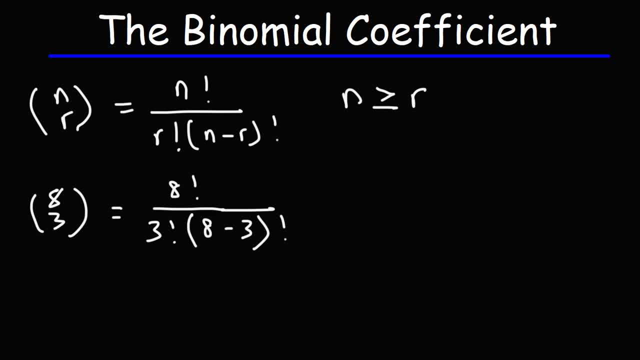 Now, how do we evaluate a factorial expression? If you saw this 4 factorial, what does that mean? 4 factorial is equivalent to this expression. It's 4 times 3 times 2 times 1.. So 4 times 3 is 12 times 2 is 24 times 1.. 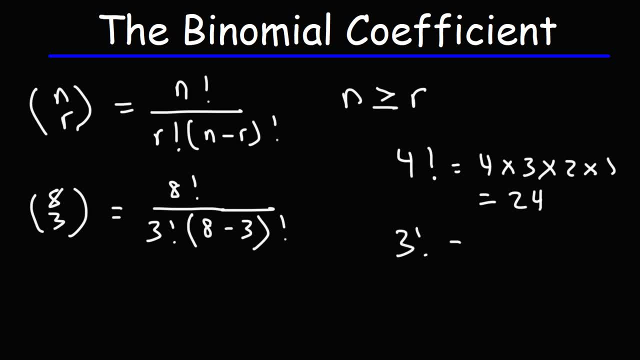 That's going to be 24.. 3 factorial is simply 3 times 2 times 1,, which is 6.. 0 factorial is 1 and 1 factorial is also 1.. So those are some things That you just need to commit to memorization. 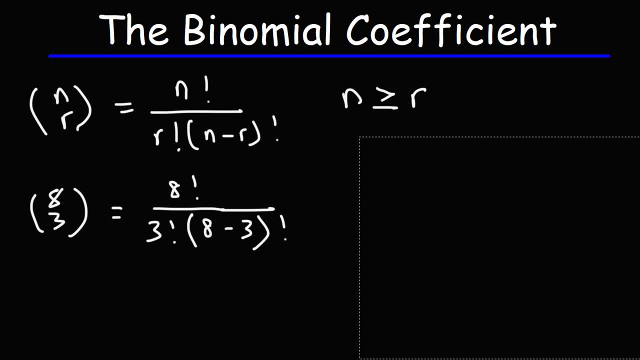 0 and 1 factorial. So, knowing that we can evaluate this expression, So we have 8 factorial over 3 factorial And then 8 minus 3, that's going to be 5.. So we have 5 factorial. 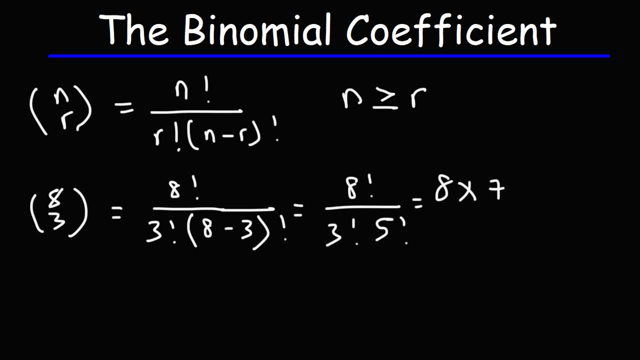 Now 8 factorial is 8 times 7 times 6 times 5 factorial, Because this will take us all the way to 1. But we don't need to go that far. Notice that we can cancel a 5 factorial. 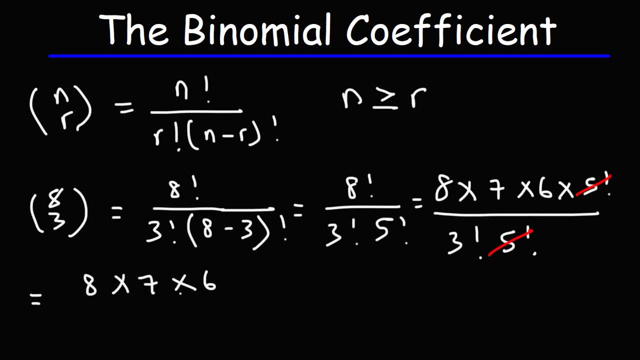 So we're left with 8 times 7 times 6.. 3 factorial. we can break that up into 3 times 2 times 1.. Now, 8 times 7 is 56.. 3 times 2 times 1 is 6.. 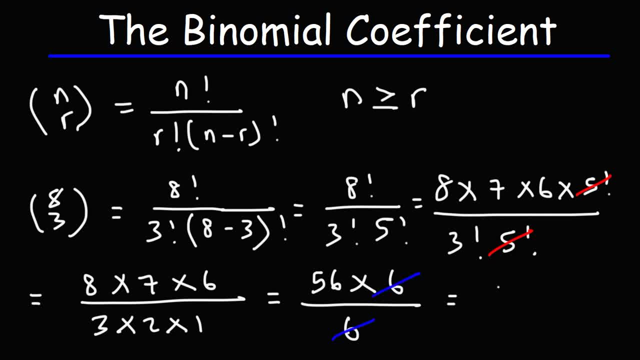 6 divided by 6 is 1.. Therefore, the final answer is going to be 56.. So that is the value of the binomial coefficient 8 above 3.. Now let's try some other examples. Try this one. 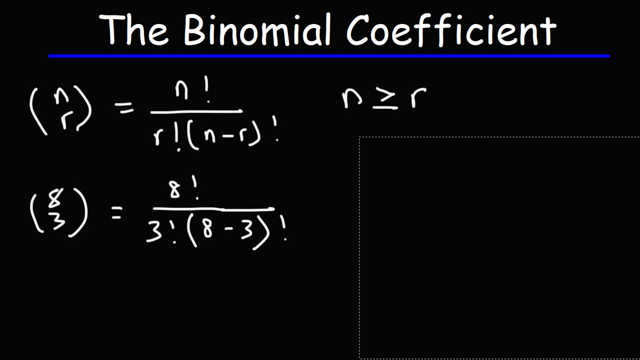 0 and 1 factorial. So, knowing that we can evaluate this expression, So we have 8 factorial over 3 factorial And then 8 minus 3, that's going to be 5.. So we have 5 factorial. 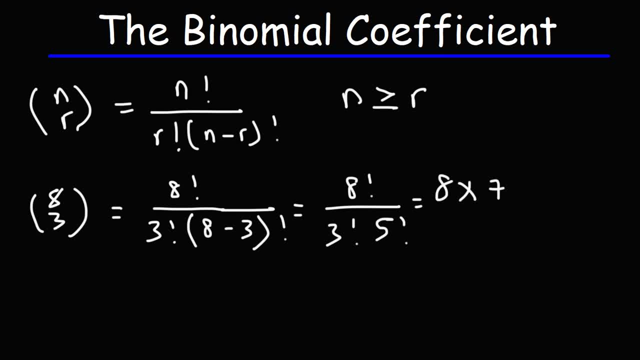 Now 8 factorial is 8 times 7 times 6 times 5 factorial, Because this will take us all the way to 1. But we don't need to go that far. Notice that we can cancel a 5 factorial. 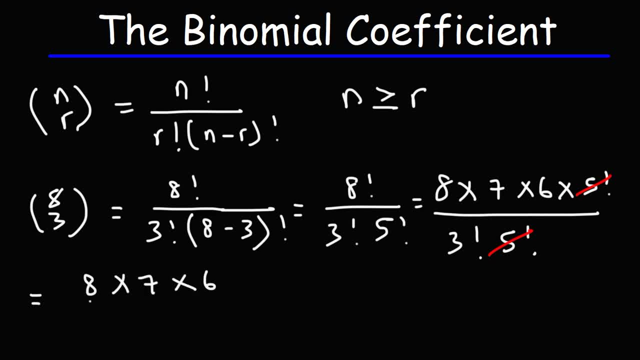 So we're left with 8 times 7 times 6.. 3 factorial. we can break that up into 3 times 2 times 1.. Now, 8 times 7 is 56.. 3 times 2 times 1 is 6.. 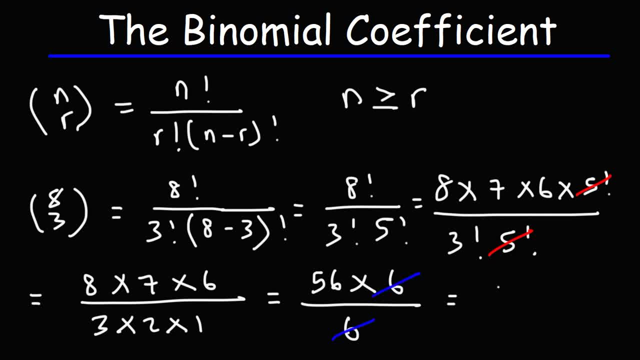 6 divided by 6 is 1.. Therefore, the final answer is going to be 56.. So that is the value of the binomial coefficient 8 above 3.. Now let's try some other examples. Try this one. 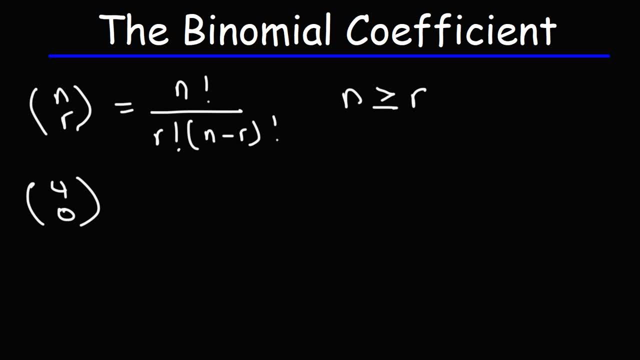 4 above 0.. Feel free to pause the video if you want to try it. In this example, n is 4.. r is 0. And then we have n minus r. That's going to be 4 minus 0.. 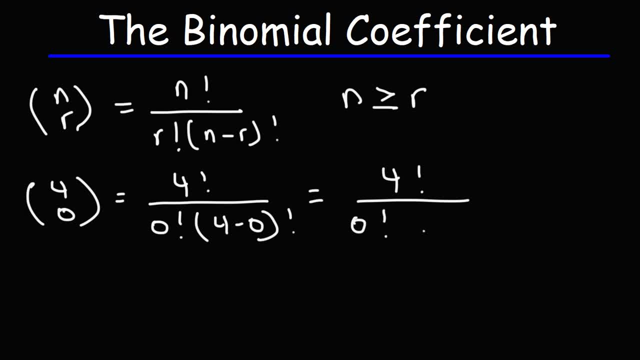 So we have 4 factorial over 0 factorial times 4 factorial. This will cancel. 4 divided by 4 is 1. 0 factorial is also 1.. So the final answer is simply 1.. So let's try this again. 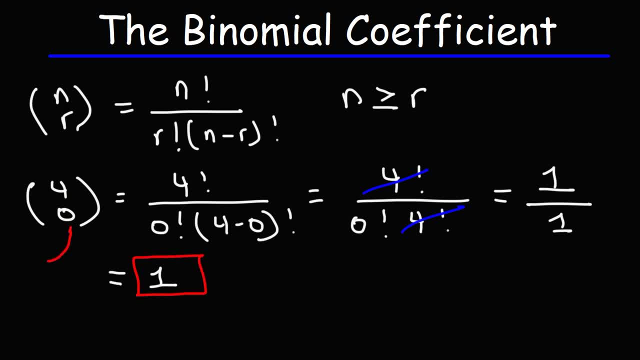 So any time you see a number, if you see a 0 on the bottom, regardless of what this number is, your final answer will be 1.. So if it's 5 above 0, 6 above 0,, 7 above 0, it's going to simplify to 1.. 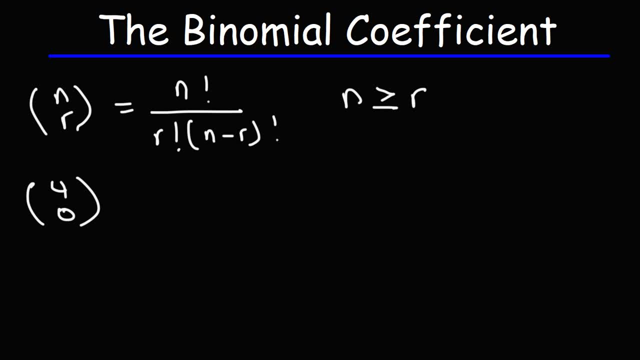 4 above 0.. Feel free to pause the video if you want to try it. In this example, n is 4.. r is 0. And then we have n minus r. That's going to be 4 minus 0.. 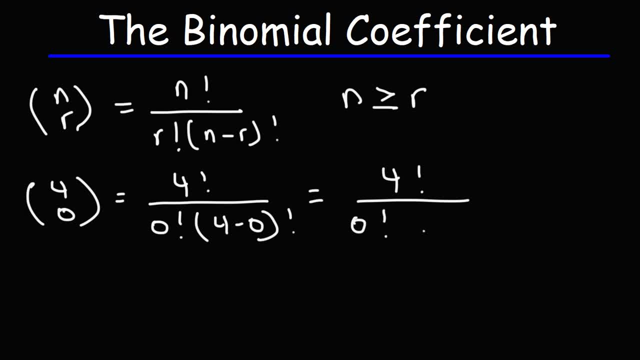 So we have 4 factorial over 0 factorial times 4 factorial. This will cancel. 4 divided by 4 is 1. 0 factorial is also 1.. So the final answer is simply 1.. So let's try this again. 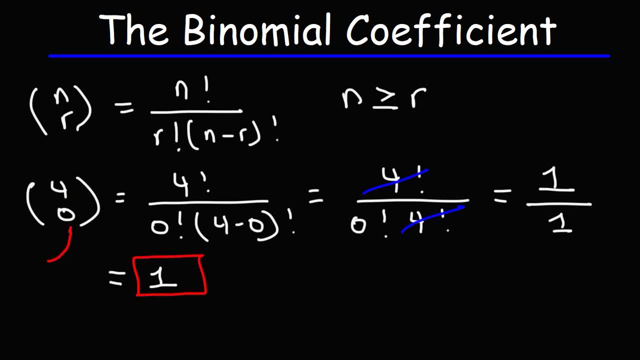 So any time you see a number, if you see a 0 on the bottom, regardless of what this number is, your final answer will be 1.. So if it's 5 above 0, 6 above 0,, 7 above 0, it's going to simplify to 1.. 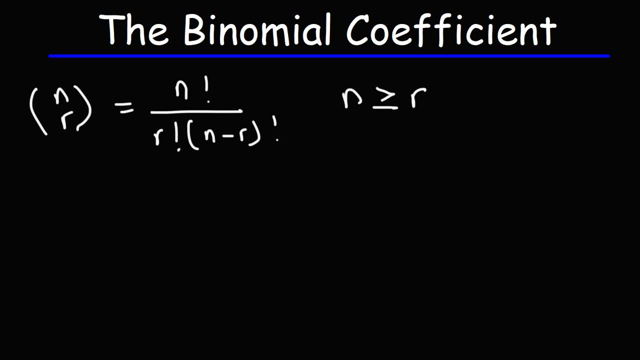 Now let's move on to the next one. Let's say we have the binomial coefficient 7 above 5.. What is that expression? equal to So n is 7.. r is 5.. And then we have n minus r factorial or 7 minus 5 factorial. 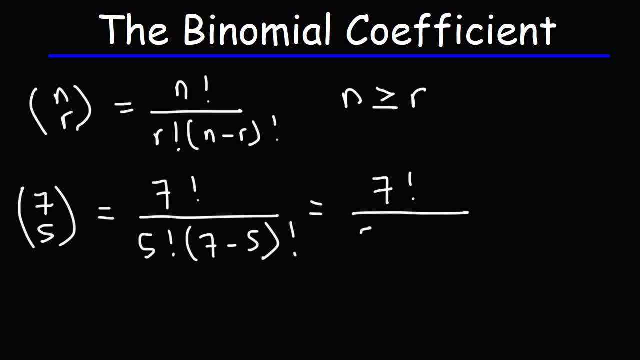 So before we expand the factorials, let's simplify what we have: 7 minus 5 is 2.. So that's 2 factorial. Now 7 factorial is 7 times 6.. Times 5, times 4, times 3, times 2, times 1.. 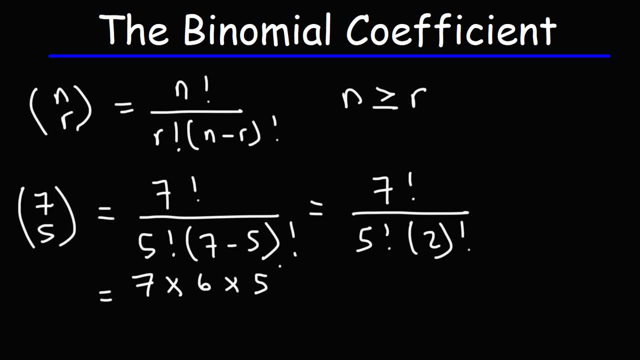 But because we have a 5 factorial here, we are going to stop at the 5 level 2 factorial. we can write that as 2 times 1.. Now let's cancel 5 factorial. 7 times 6 is 42.. 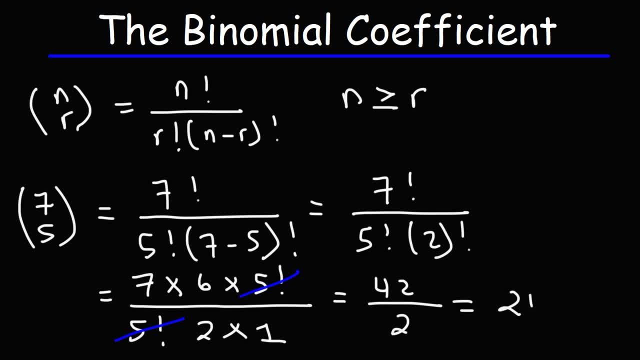 2 times 1 is 2., And then half of 42 is 21.. So that's the value of the binomial coefficient 7 above 5. It's equal to 21.. Now let's move on to another example. 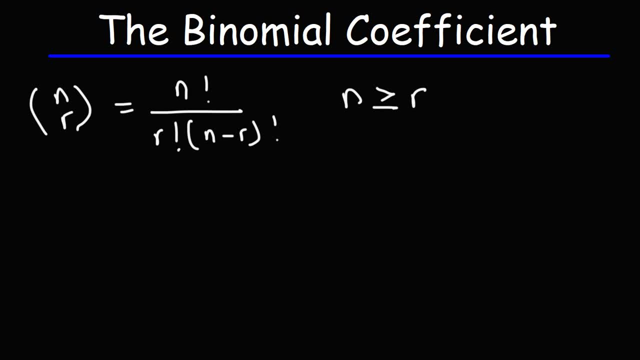 Now let's move on to the next one. Let's say we have the binomial coefficient 7 above 5.. What is that expression? What is that expression? equal to So n is 7.. r is 5.. And then we have n minus r factorial, or 7 minus 5 factorial. 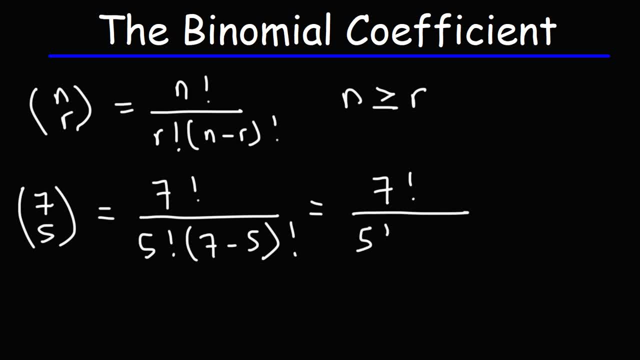 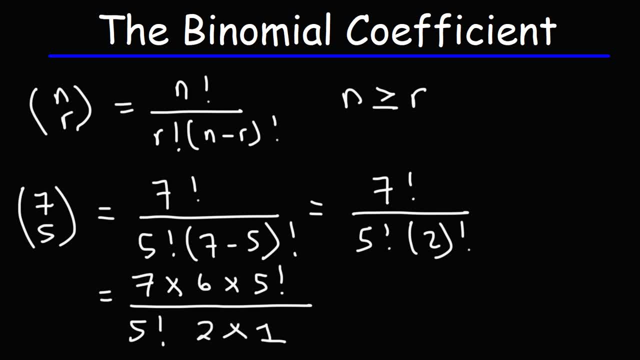 2 factorial. we can write that as 2 times 1.. Now let's cancel 5 factorial. 7 times 6 is 42.. 2 times 1 is 2.. And then half of 42 is 21.. 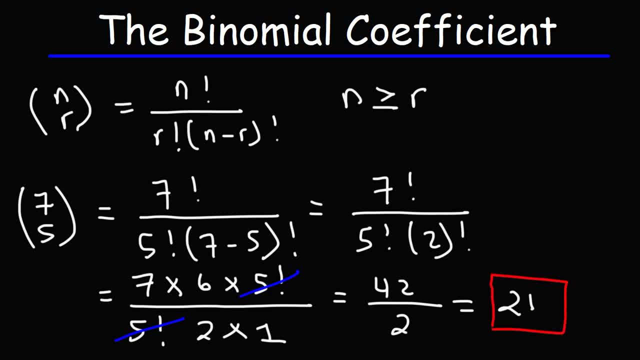 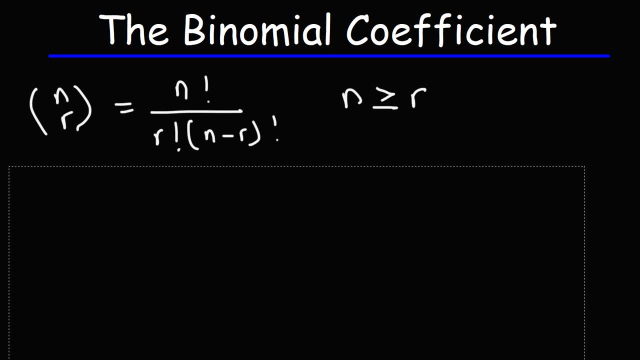 So that's the value of the binomial coefficient: 7 above 5. It's equal to 21.. Now let's move on to another example. Let's say we have this: We have a binomial coefficient where n and r are the same. 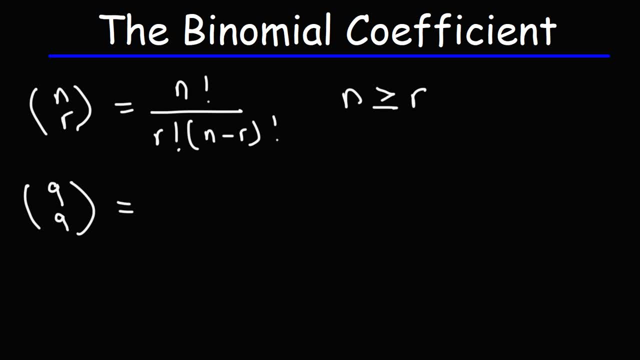 What's the value for this one? When n and r are the same, or when r is 0,, you're going to get 1.. So in this example, n is 9, r is 9.. And then n minus r, that's 9 minus. 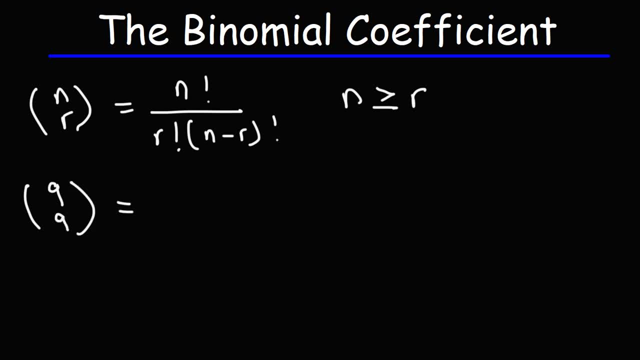 Let's say we have this: We have a binomial coefficient where n and r are the same. What's the value for this one? When n and r are the same or when r is 0, you're going to get 1.. 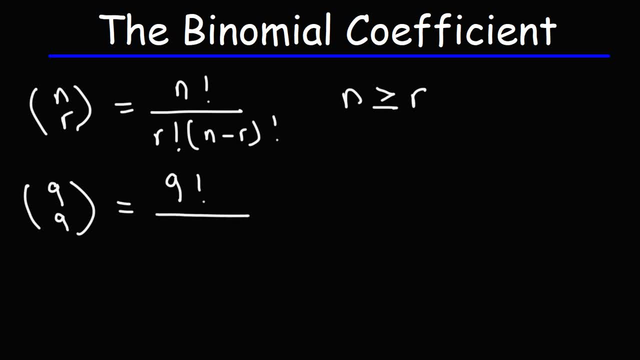 So in this example n is 9, r is 9.. And then n minus r, that's 9 minus 9.. 9 factorial we can cancel. 9 divided by 9 will give us 1.. And then 9 minus 9 is 0. 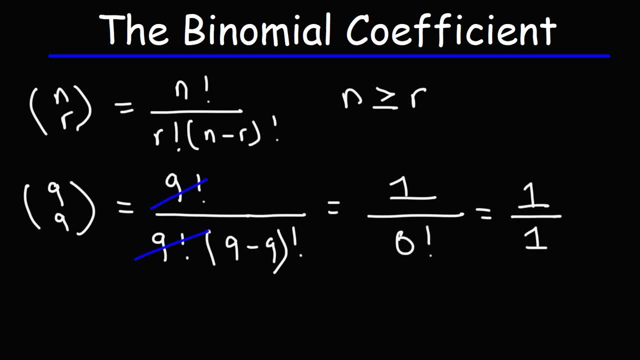 So we have 0 factorial. 0 factorial is 1.. 1 divided by 1 is 1.. So, as a shortcut, just remember: if n and r, if they're identical, it's going to equal 1.. 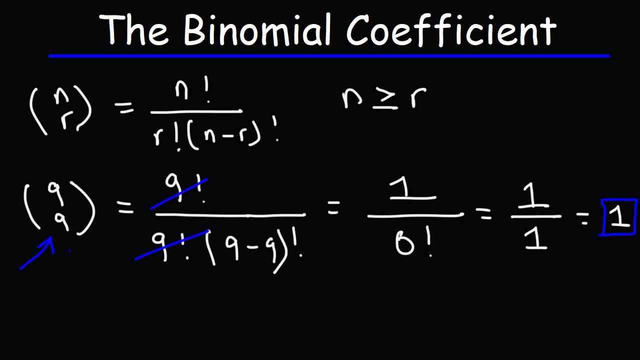 Or if r is 0, you're going to get 1 as well. Now let's see what happens when n is just 1 unit above r. Go ahead and look at this. Go ahead and look at this. Go ahead and try these two. 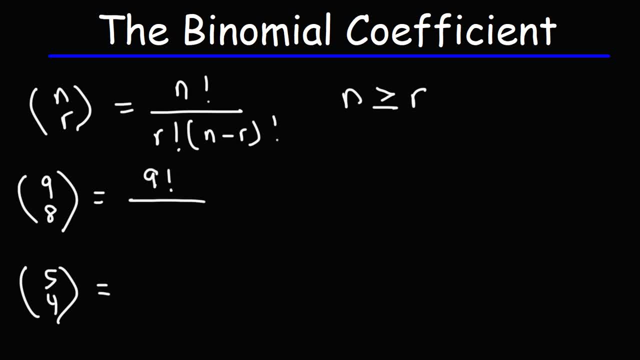 So this is going to be 9 factorial over 8 factorial times 9 minus 8 factorial. 9 factorial is going to be 9 times 8 factorial And 9 minus 8, that's going to be 1.. 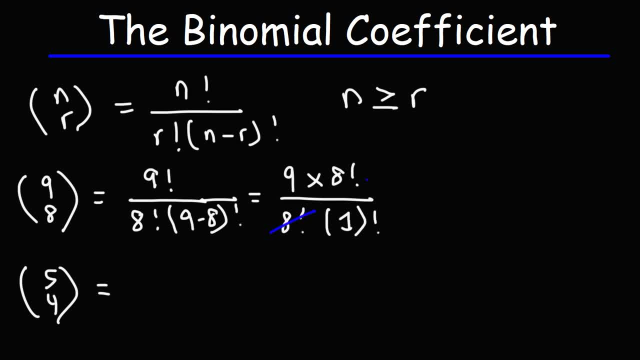 So we have 1 factorial. 8 factorial is going to be 1.. 8 factorial is going to be 1.. 8 factorial will cancel. We get 9 over 1 factorial is 1.. So we just get 9.. 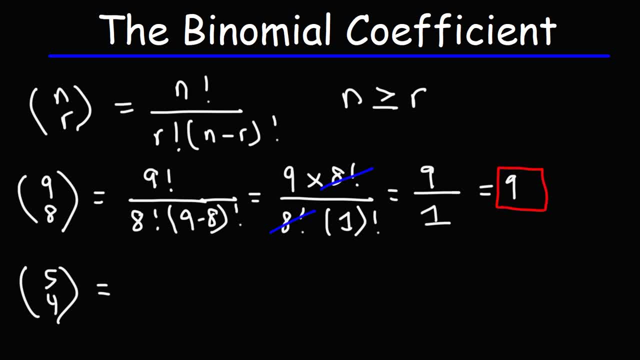 Notice that when n is 1 unit above r, we're going to get n, Whatever n is. So here 9 is 1 unit above 8. So in this case we just get 9.. Let's see that for the next example. 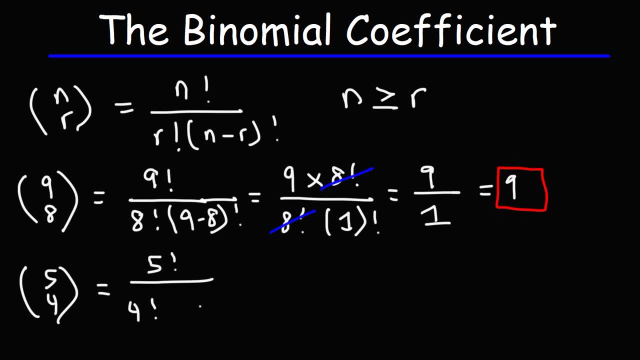 So n is 5.. r is 4.. 5 factorial is 5 times 4 factorial And 5 minus 4 is 1.. So now we can cancel 4 factorial And we're going to get a similar situation. 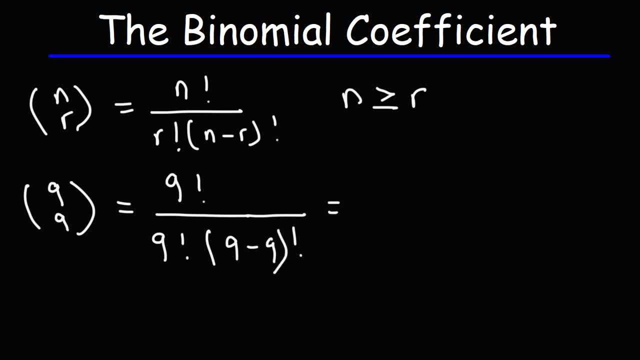 9 factorial. we can cancel: 9 divided by 9 will give us 1.. And then 9 minus 9 is 0.. So we have 0 factorial. 0 factorial is 1.. 1 divided by 1 is 1.. 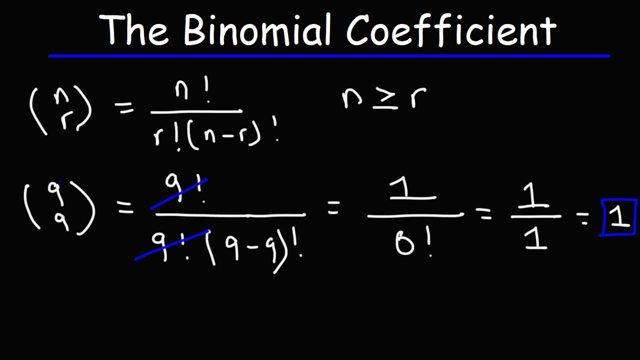 So, as a shortcut, just remember: if n and r, if they're identical, it's going to equal 1.. Or if r is 0, you're going to get 1 as well. Now let's see what happens when n is just 1 unit above r. 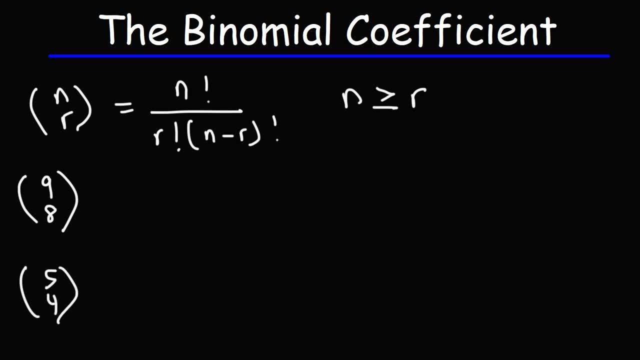 Go ahead and try these two. So this is going to be 9 factorial over 8 factorial Times, 9 minus 8 factorial. 9 factorial is going to be 9 times 8 factorial And 9 minus 8, that's going to be 1.. 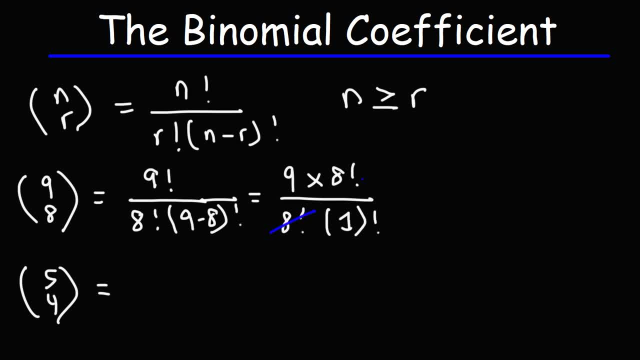 So we have 1 factorial. 8 factorial will cancel. We get 9 over 1. factorial is 1.. So we just get 9.. Notice that when n is 1 unit above r, we're going to get n, whatever n is. 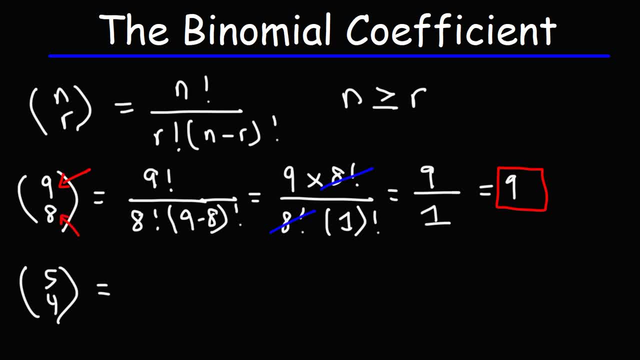 So here 9 is 1 unit above 8.. So in this case we just get 9.. Let's see that for the next example. So n is 5, r is 4.. 5 factorial is 5 times 4 factorial. 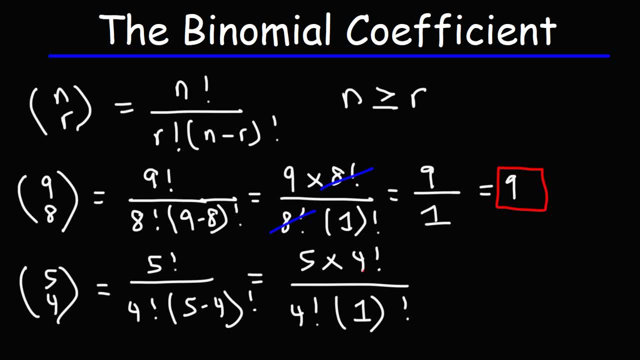 5 minus 4 is 1.. So now we can cancel 4 factorial And we're going to get a similar situation: We're going to get 5.. So, just like in the previous example, we see that n is 1 unit higher than r. 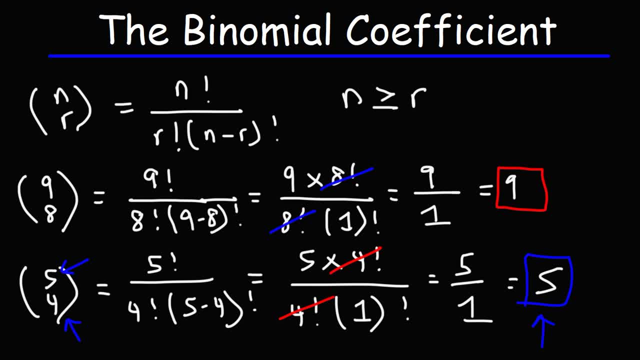 And our answer is equal to n. So that's basically it for this video. So now you know how to evaluate a binomial coefficient. All you have to do is use this formula And then simplify the expression that you get. Thank you.